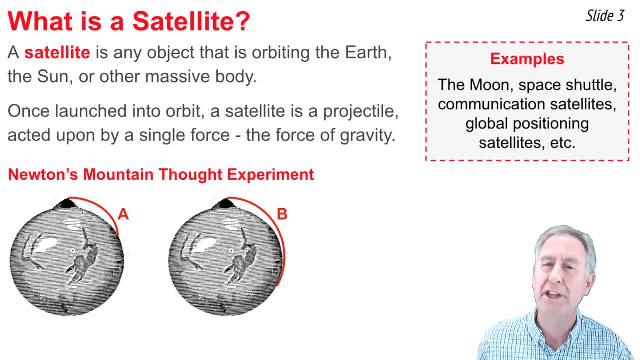 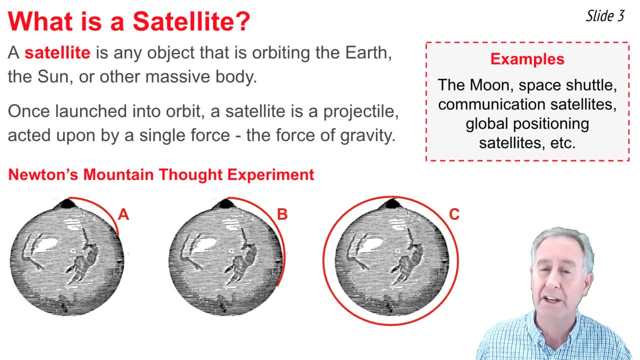 it finally fell and struck the Earth. He imagined that there could be such a speed that you could fire the cannonball at that. it would fall towards the Earth but never land on the Earth. Relative to the straight-line tangent path, at every point along its trajectory it would begin to fall but never touch the Earth. 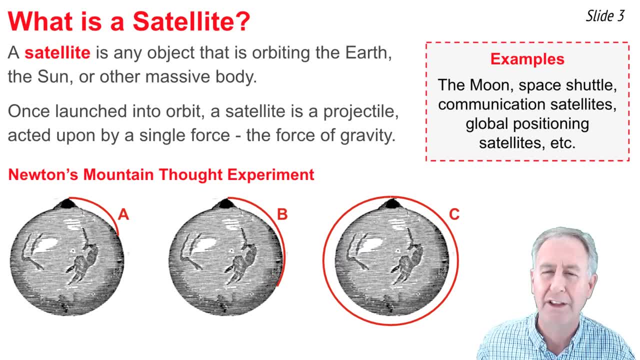 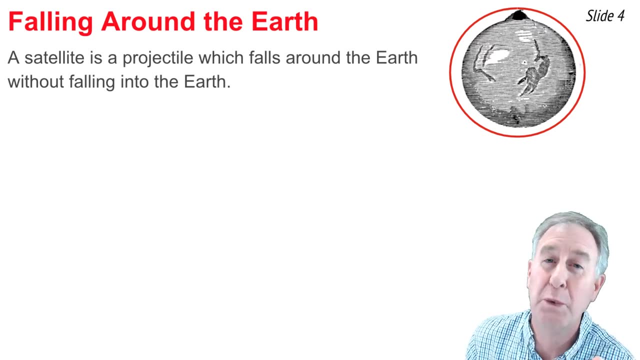 because its curvature matched the curvature of the Earth. And then he imagined that you could fire it a little faster still, and such a cannonball would make an elliptical path, a circular path around the surface of the Earth. Newton's mountain thought experiment teaches us that a satellite is a projectile that falls. 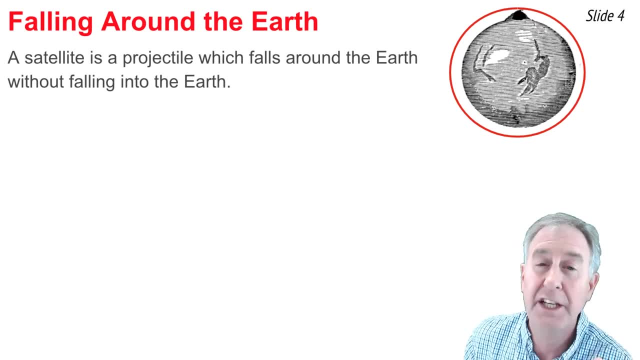 around the Earth without ever falling into the Earth. To illustrate the idea, consider this projectile launched horizontally from the position of the red dot. In the absence of gravity, this projectile would travel tangent to the Earth and end up at location 1, prime. 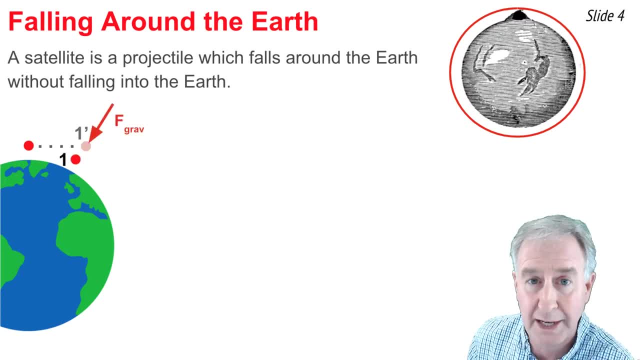 But because of the influence of gravity pulling it downwards, instead it's at location 1 and traveling tangent to the circular path Some time later. this projectile, in the absence of gravity, would be located at position 2, prime, But because of the influence of gravity pulling it downwards, it's located at position 2. 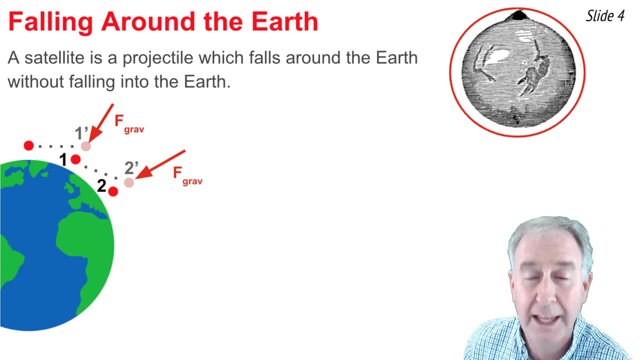 instead again traveling tangent to the circular path, And because of that, some time later, in the absence of gravity, it would be located at position 3, prime. But again gravity pulls it downwards and it's located at position 3 instead and a traveling tangent to the circular path. 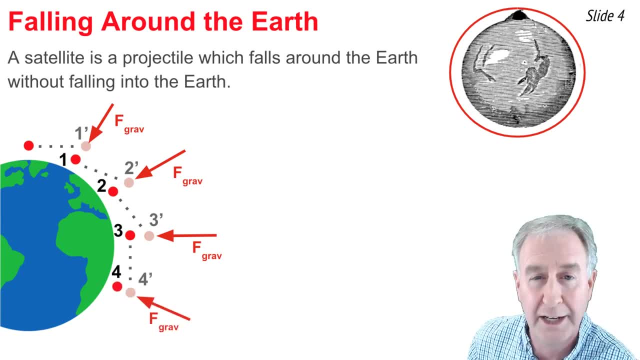 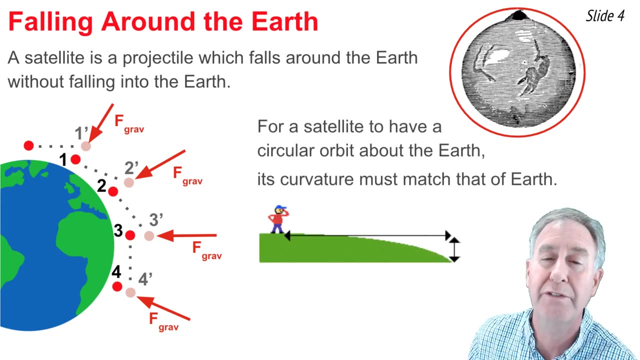 Now this thought experiment could continue, and what we have is a projectile that is launched horizontally at such a high speed that it falls towards the Earth, but never falls into the Earth. In order to have a satellite make a circular path around the Earth, its curvature must match the curvature of the Earth. 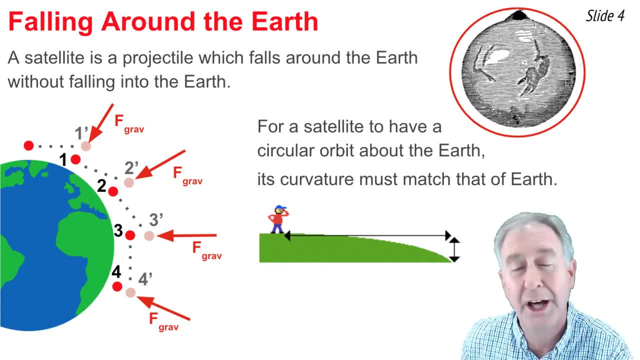 If you were to stand on Earth's surface and look out horizontally along the surface of the Earth, you would note that for every 8,000 meters horizontally, the Earth curves downwards 5 meters. The significance of 5 meters is that's the distance that a projectile falls in one second. So if you 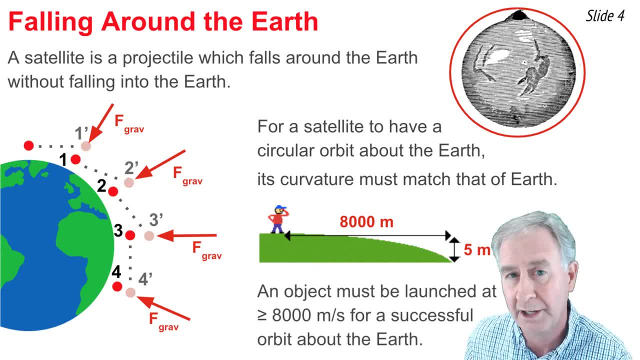 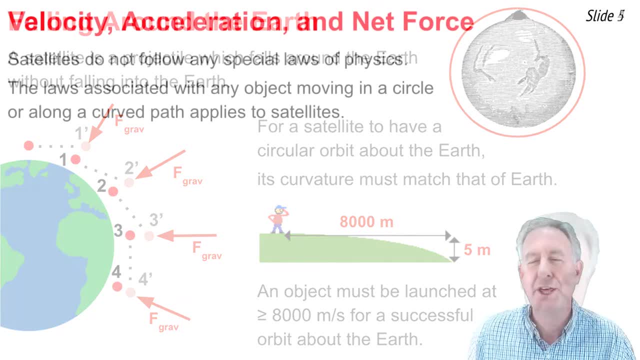 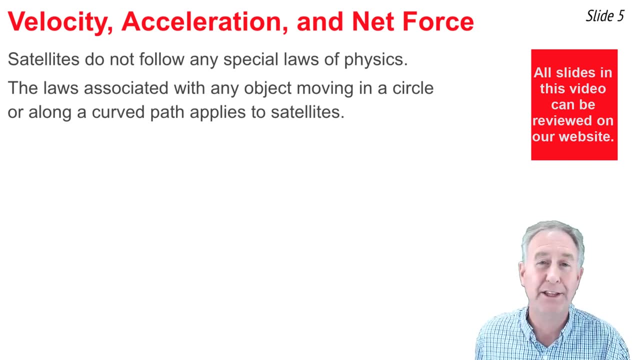 could shoot a projectile that travels 8,000 meters horizontally in one second. it would fall downwards towards the Earth, but never touch the Earth. There are no special laws of physics that apply just to satellites. Instead, the very laws that apply to any object that's moving in. 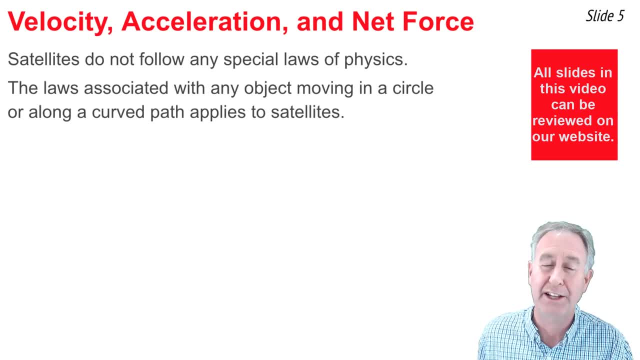 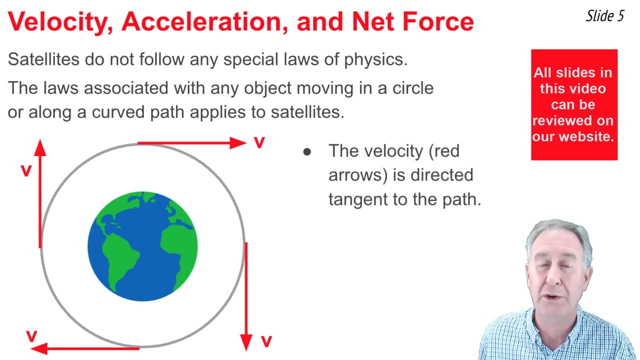 a circle or along a curved path also applies to satellites. Some of those laws have to do with the velocity, acceleration and net force. Here is a diagram of an Earth-orbiting satellite orbiting in a circular path And at every location along the circle the direction of the velocity vector. 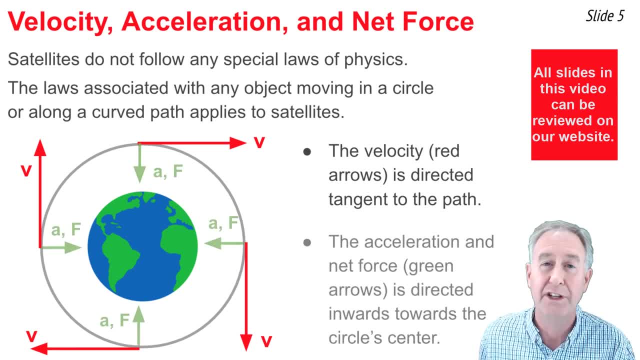 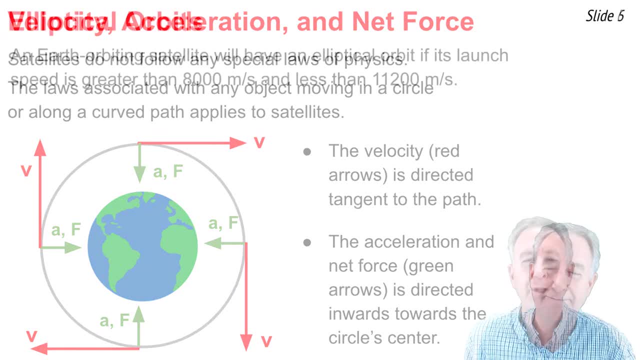 is directed tangent to the circle and the direction of the acceleration and net force vectors are perpendicular to the path and directed towards the center of the Earth. When an Earth-orbiting satellite is put into orbit at 8,000 meters per second, it travels around the 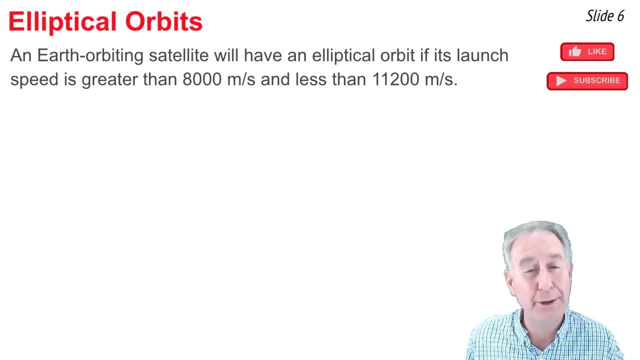 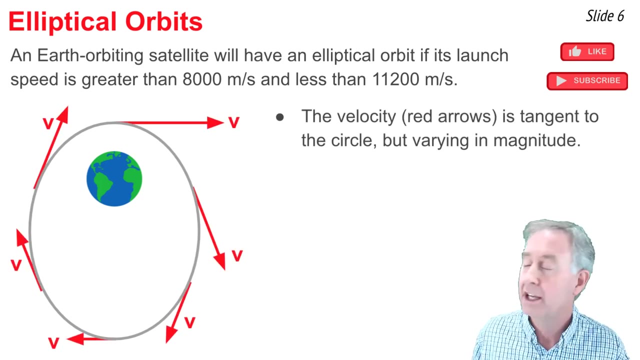 Earth in a circular orbit, But if launched with a speed greater than 8,000 meters per second and less than about 11.2 kilometers per second, our Earth-orbiting satellite will orbit with an elliptical path. as shown At every location along that path, the direction of the velocity vector: 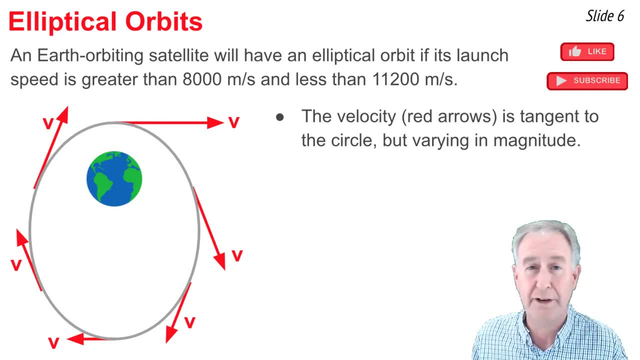 is tangent to the path, But the magnitude of the velocity vector is constantly varying. As you'll note here, the magnitude is greatest when the satellite is closest to the Earth and the velocity is smaller. The velocity vector is constantly varying. The magnitude of the Earth is 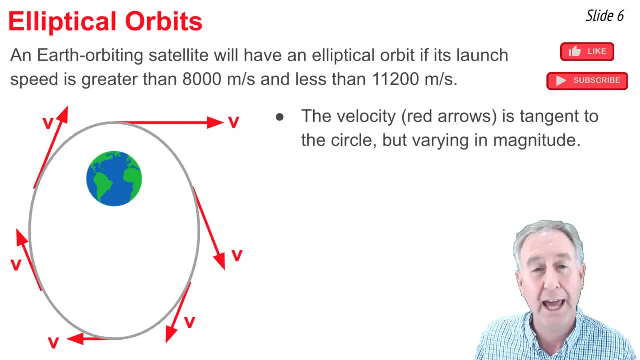 greater when the satellite is closest to the Earth, and the velocity is smaller. The magnitude of the satellite is greatest when the satellite is furthest from the Earth. As for the acceleration and net force vectors, those are gravity-influenced vectors, and so they're always directed towards. 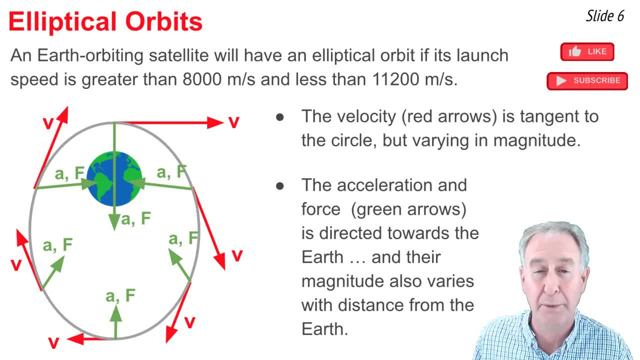 the center of the circle. at all points along the pathway of this elliptical orbit, The direction is always inward, but the magnitude is varying, as you'll see in the diagram, and influenced by the law of universal gravitation When the satellite is closest. 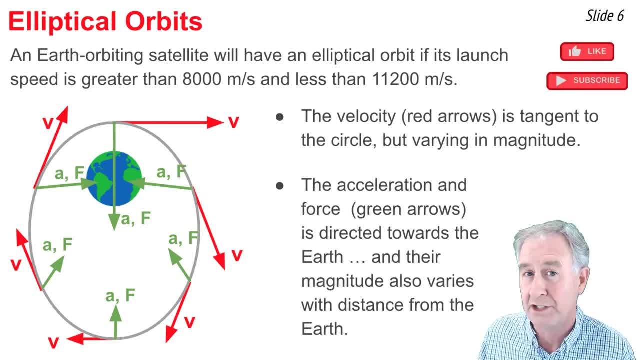 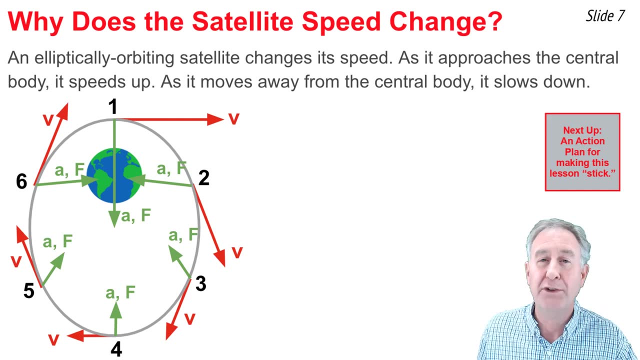 to the Earth, the force of gravity and the acceleration that it causes is the largest, and when the satellite is furthest from the Earth, the force of gravity and the acceleration it causes is the smallest. An elliptically orbiting Earth satellite is changing its speed As it travels along the orbital path from location 4 to location 1,. 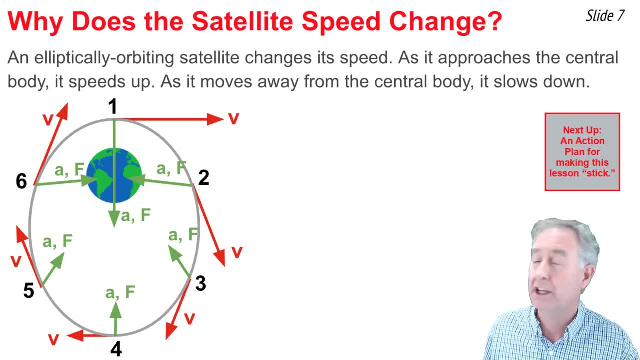 it's increasing its speed and, as it travels along its elliptical path from location 1 to location 4, it's decreasing its speed. But why? Why would a satellite change its speed? Well, one quick and incorrect answer would be to say it's changing its speed in the way it does.